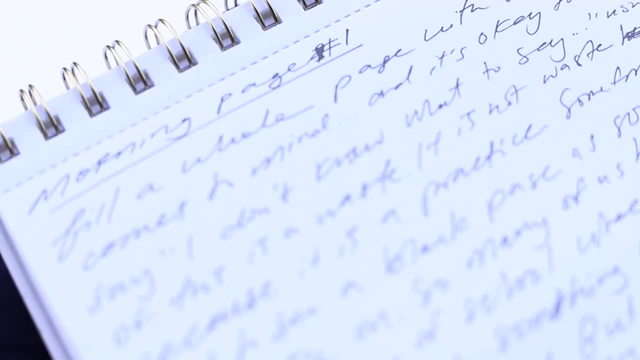 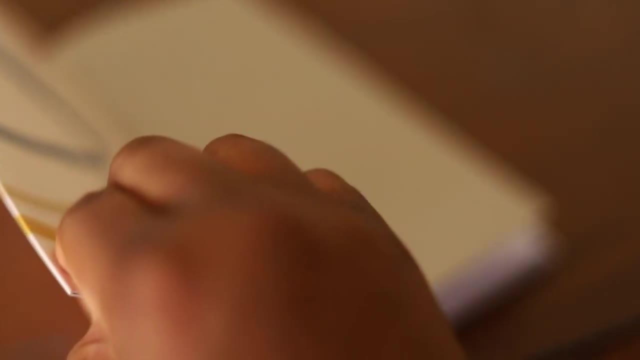 and write poetry, prose, music and more. This exercise is designed to help you break out of writer's block or simply be inspired to write and finally fill out one of those blank pages inside of your journal. So if you need to pause this video to go and grab a journal, now is the. 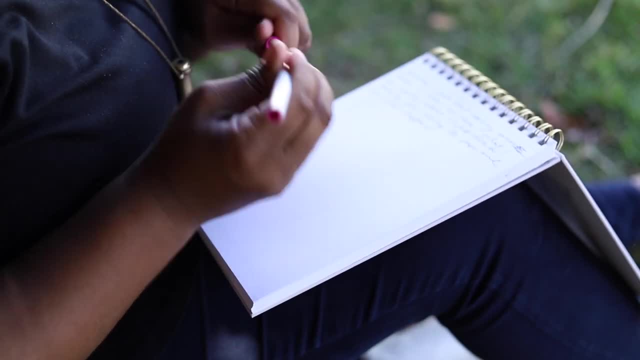 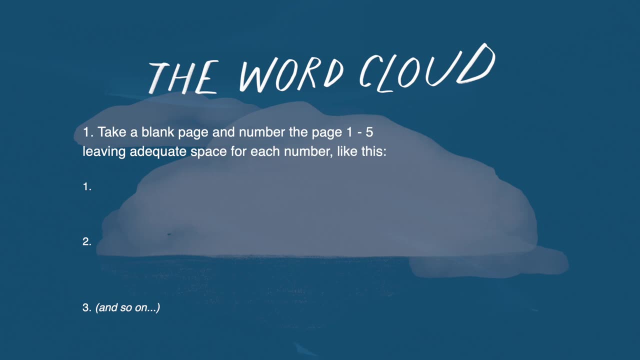 time, Or you can just use a notes app on your phone. Here are the steps to get started. Number one: take a blank page and number the page one through five, leaving adequate space between each number. In a moment, a series of words are going to fade in and out of the word cloud. During that, 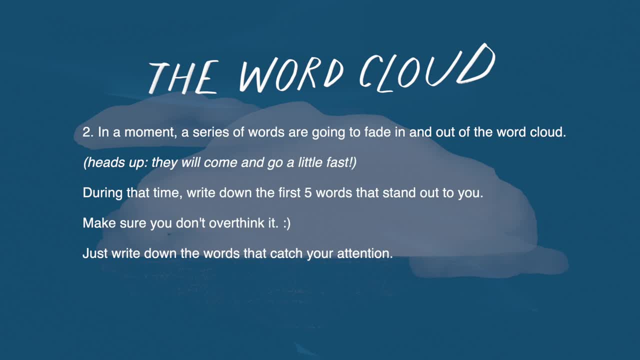 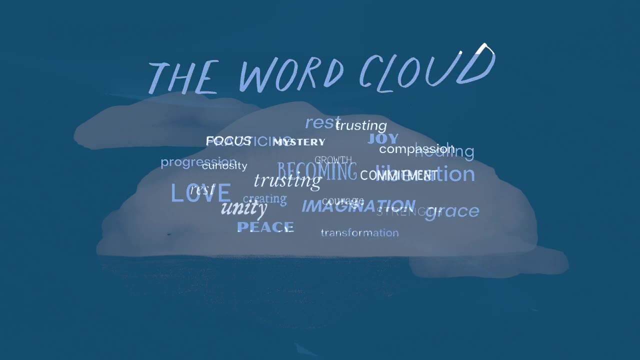 time. write down the first five words that stand out to you- and make sure you don't overthink it- and just write down the words that catch your attention. So, whenever you're ready, here are the words: Great work. One of the best things that we can do as writers is to simply pay attention. 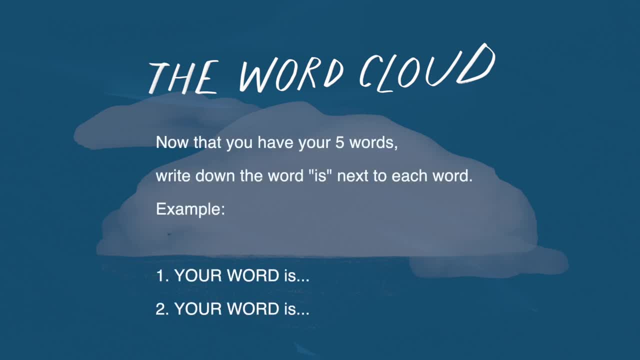 and you have done just that. So if you have five words write down, the word is next to every single word. Now I am going to show you a series of new words. Pick five more words and write them. on the other side of the word is: 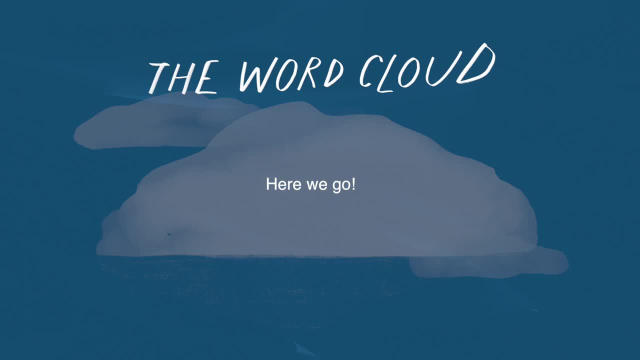 Now that you have selected these words, you now have these phrases, these statements, Which one stands out to you the most? Which one do you agree with or disagree with? Which one do you like the most? Which one do you dislike the most? Which one do you hate the most? Which one do you? 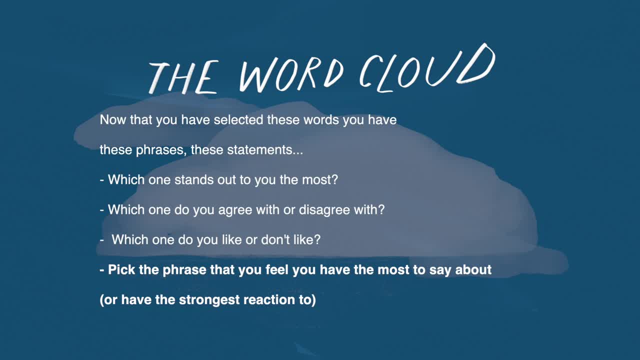 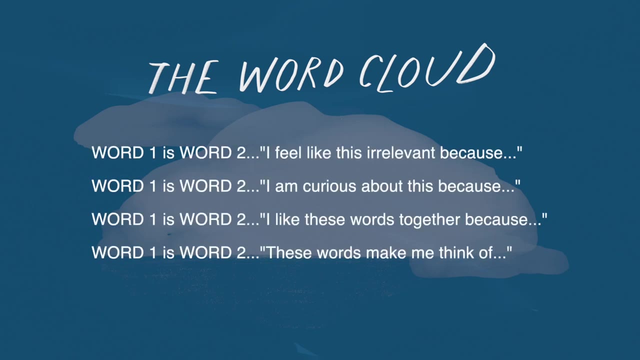 like or don't like. Pick the one that you feel that you have the most to say about. even if you really don't like it and you feel like it is silly or irrelevant, That is still something you can write about. You can literally start with the words: I feel like this is irrelevant.